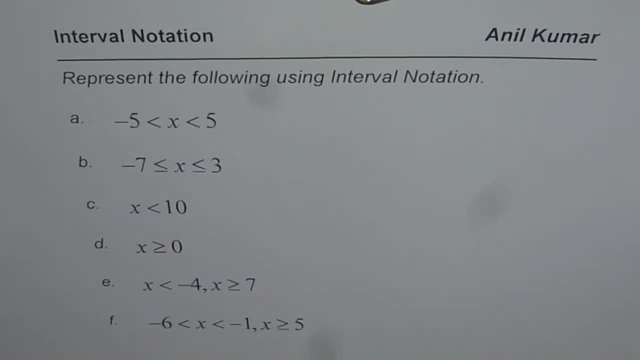 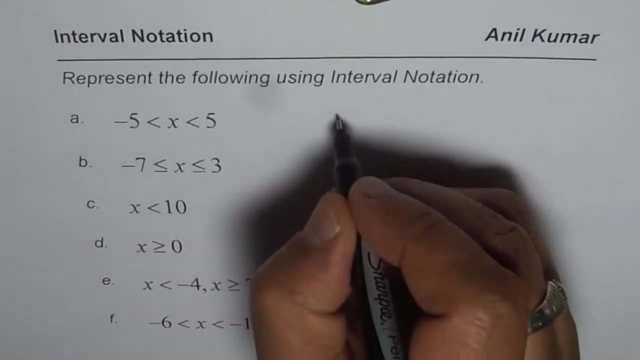 So these are the intervals given as an inequality. You can pause the video. write them in interval notation. Here is the solution: When I say x is between minus 5 and 5, where both are not included, we'll write it as minus 5.. 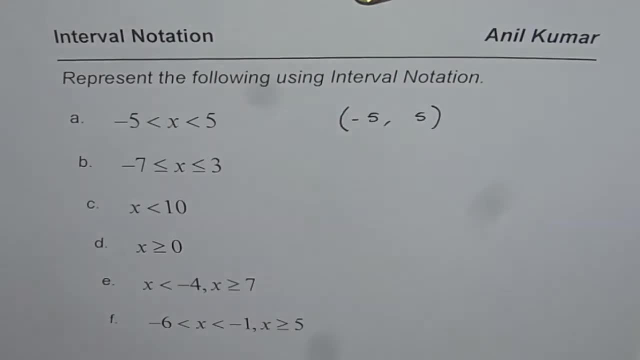 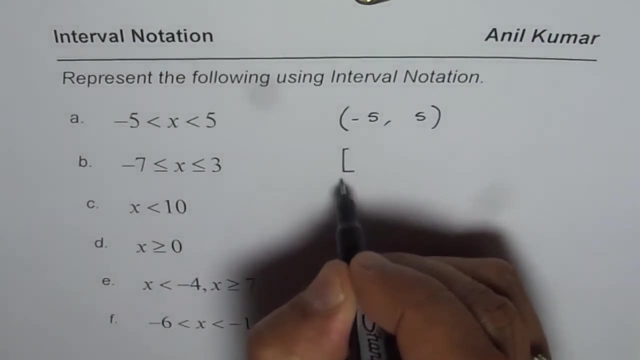 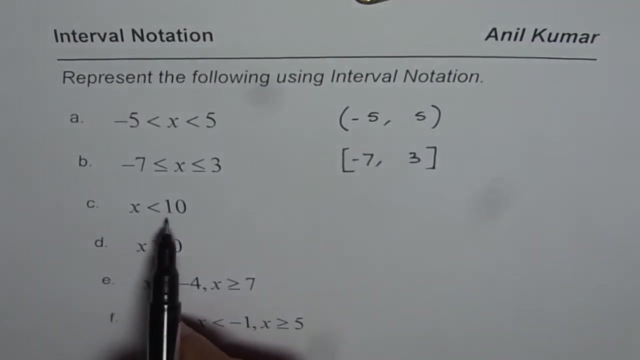 So minus 5 to 5, both not included. In the second case, minus 7 and 3 are included And therefore we'll use these brackets, which are the square brackets. So use square brackets Now we have. x is less than 10.. 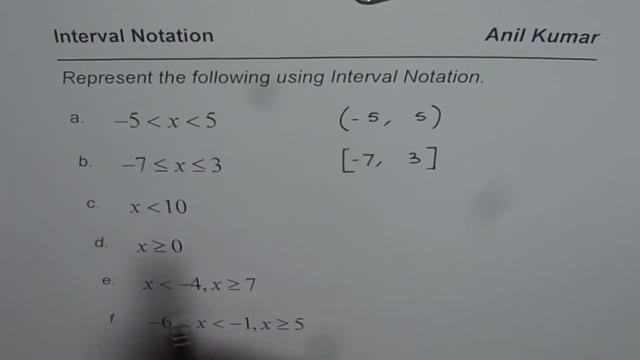 Less than 10 means it could go up to negative infinity, which can never be included. So it is negative infinity to 10.. 10 is also not included, so open bracket. Then we have: x is greater than equal to 0.. Greater than equal to means square bracket. 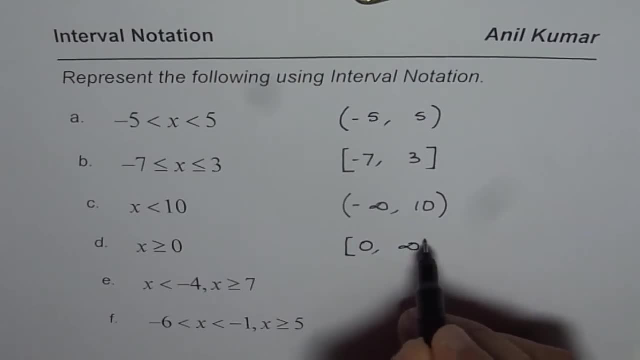 starting from 0 up to infinite, which should not be included. Now we have a slightly complicated situation. x is less than minus 4. That means it will go to minus infinity, right? So this is not equal to. And now, when we use comma, we could. 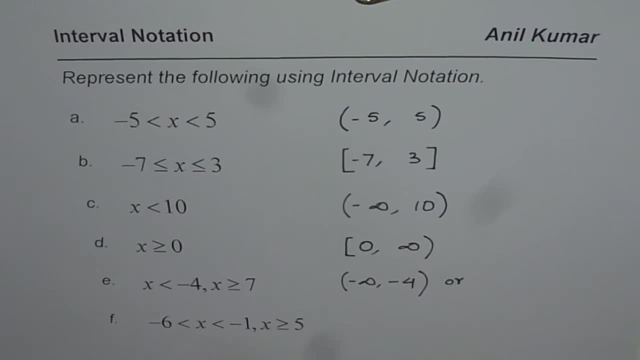 use OR. We could use OR, So. these are two examples of disjunctions: OR. You could also use union, So I'll use union in this case. And then we have: x is greater than equal to 7, which means 7 is. 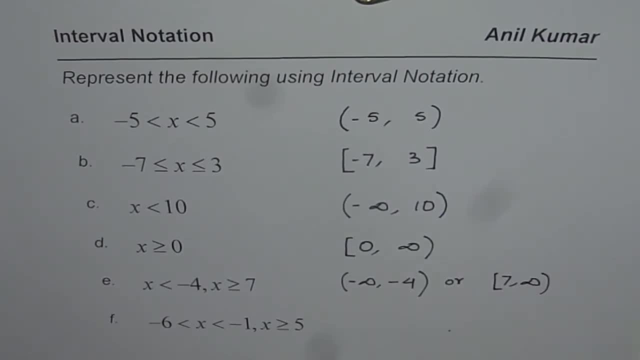 included and go to infinity. So OR this, Or we could, as I said, use union, which I'm going to do here now. The last example, x, is between minus 6 and minus 1.. Both are not included, So it is kind of like this union. 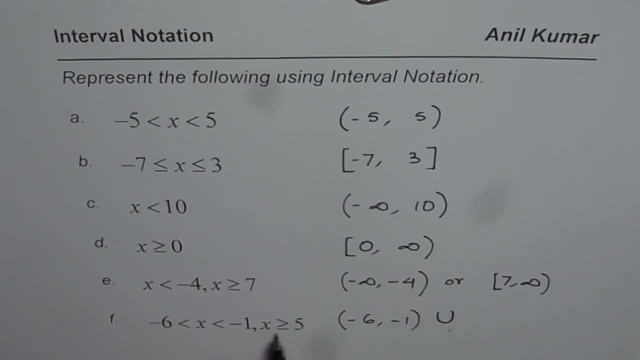 which is same as, OR is same as or. x is greater than equal to 5, in this case also, 5 is included, and it is kind of going up to infinity, right, And infinity should never be included. So that is how you can represent these inequalities, in the form of interval notation. I hope that. helps, Thank you.